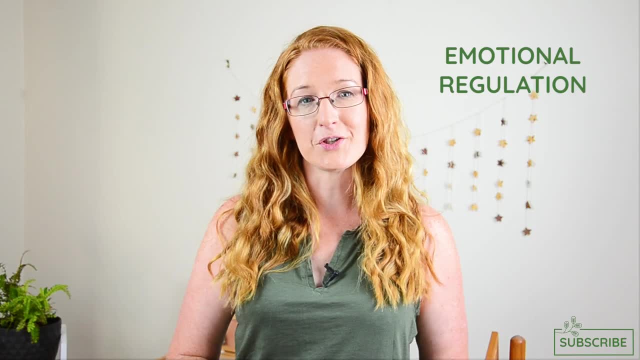 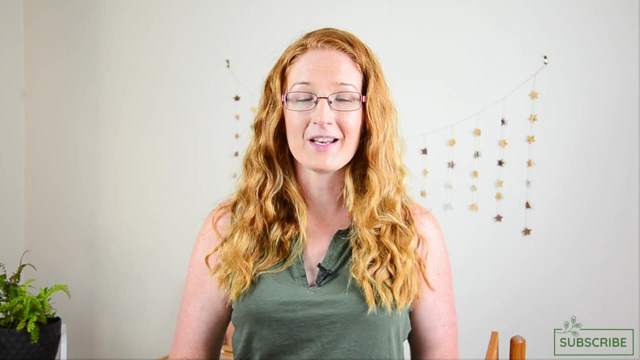 materials that you can buy from the shops. The second is that they're learning emotional regulation and the ability to learn how to control the environment. So they're learning to let things go. So, of course, going and having to put their beautiful artworks in the compost bin. 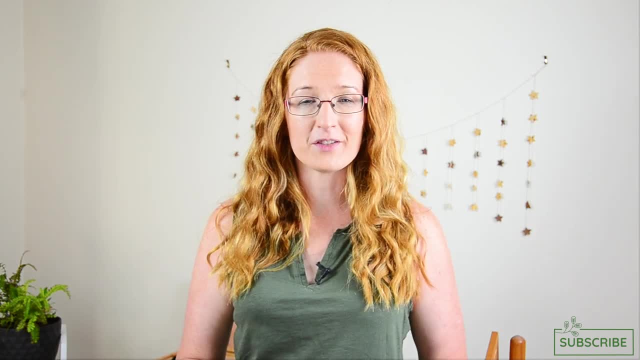 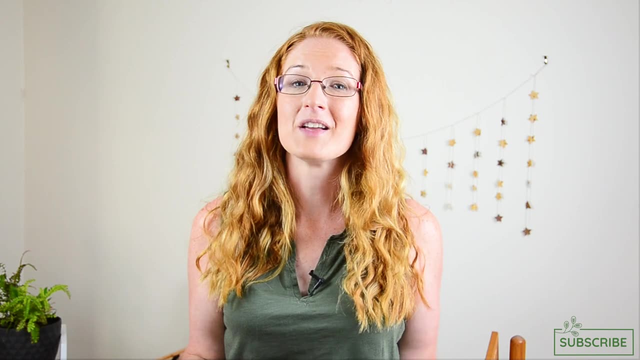 can feel uncomfortable and sad and there's going to be a whole bunch of emotions and it's really just talking to them and saying that those emotions are completely normal, but we can't keep it because it's starting to die. And the third is that they are learning when we take 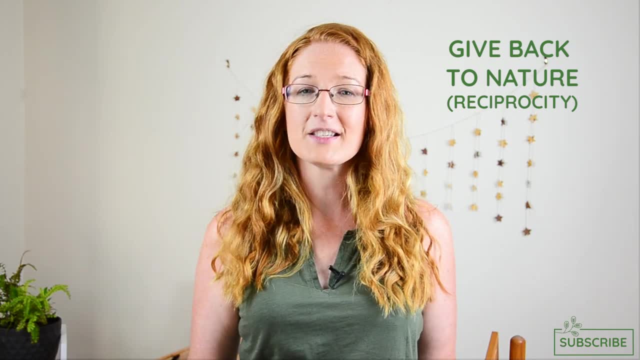 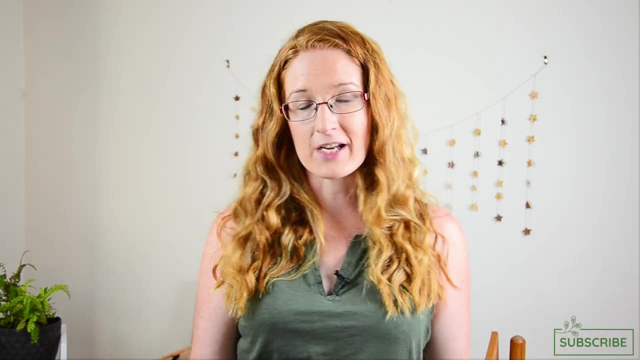 from nature, that we have to give it back to nature, and that's a really great lesson to learn, because that's how the world works. We need to use resources and then we need to give them back and reuse those resources. If you're enjoying this video, please give it a like and, if you would like, 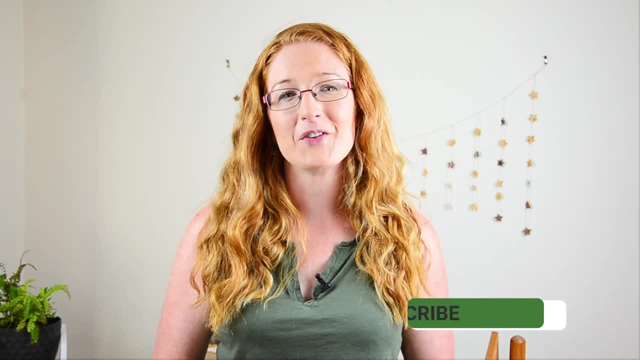 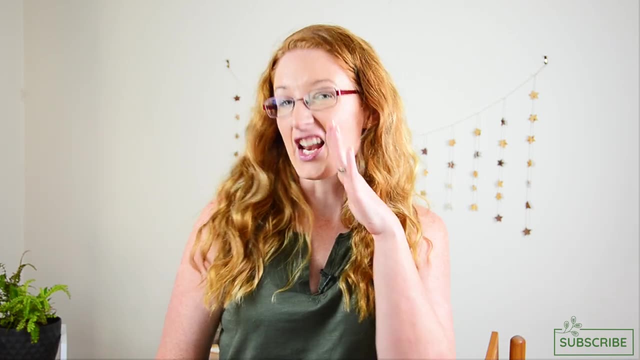 more nature, craft tips and tricks, or just to get your kids outside more often. please subscribe and click the bell to be notified every time I make a new video. If your child has never had to throw their artwork away and you've resorted to throwing it in the bin when they're not looking, it may be a. 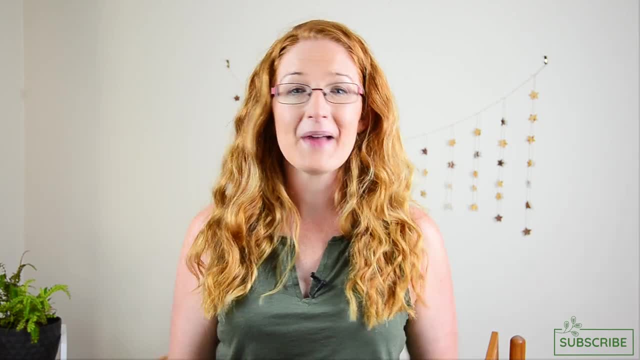 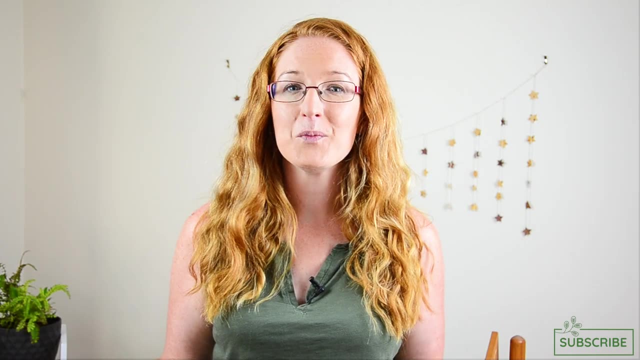 challenge at first to do this activity, but nature is an amazing teacher and talking about what is going to happen to the nature craft is a fantastic place to start with a conversation By asking them what they've seen leaves and flowers do when they're picked off the stem. what do they think? 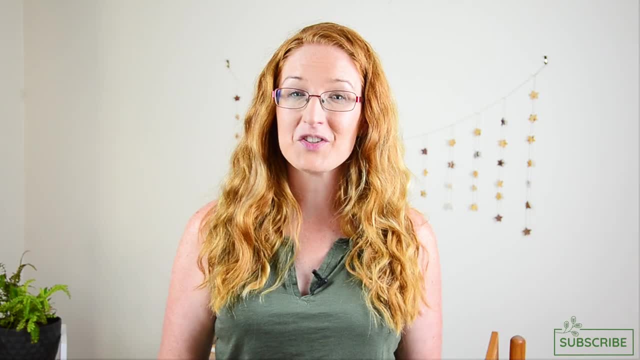 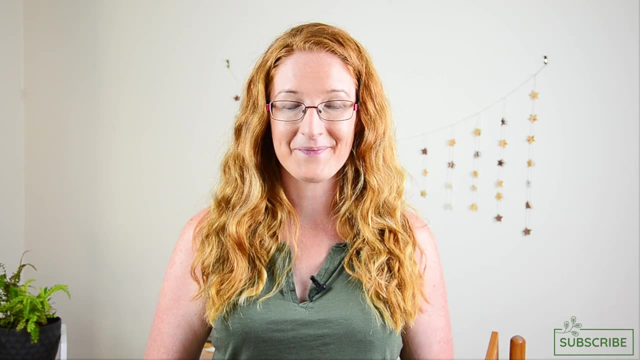 will happen to the artwork over time. if they understand that the materials will die and curl, you might like to suggest that they take a photo of it so they can remember what it looked like on the first day they made it To extend on this activity. they can take a photo of it every single. 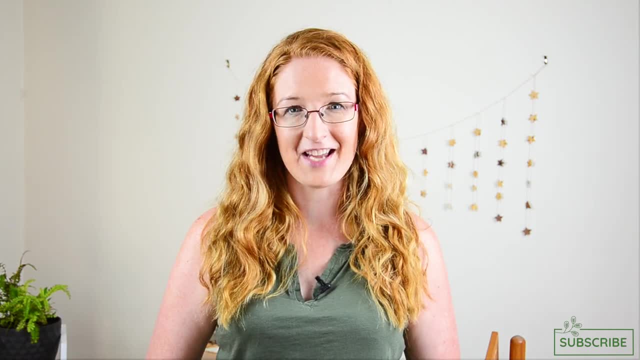 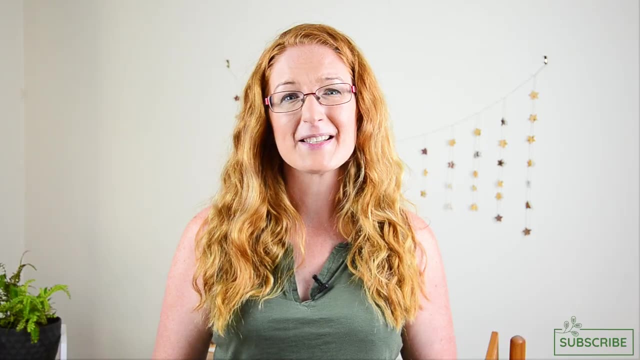 day and look back and see and discuss how it has changed every day. It's actually a really lovely activity to do together. When you get to the day that you need to retire the nature craft because you know bits and pieces are falling off the page, then an open discussion about the rhythm of taking 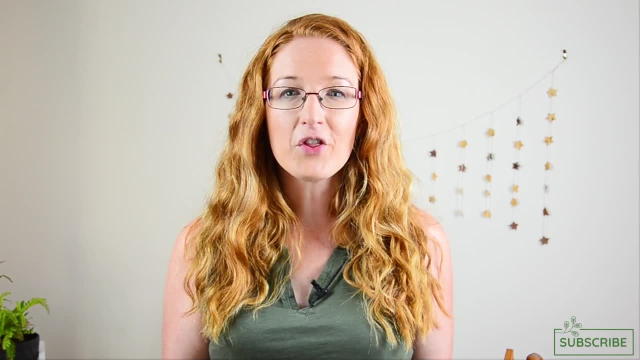 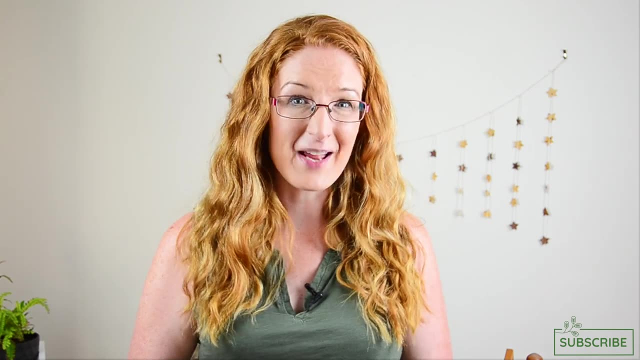 and giving back to nature can really help Now that we've gotten through that. there are nature crafts that you can make and will last for so much longer than you think. but, as mentioned before, it can really depend on several things: The materials, the glue that are used and the environment. 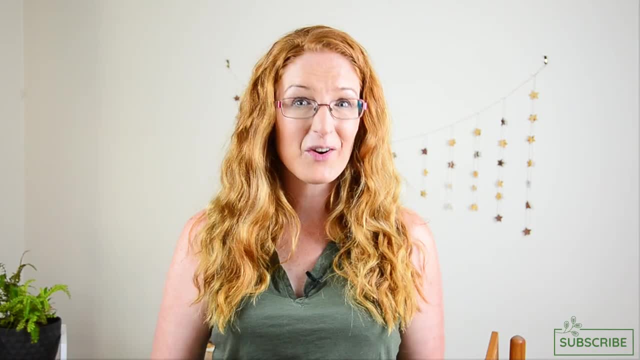 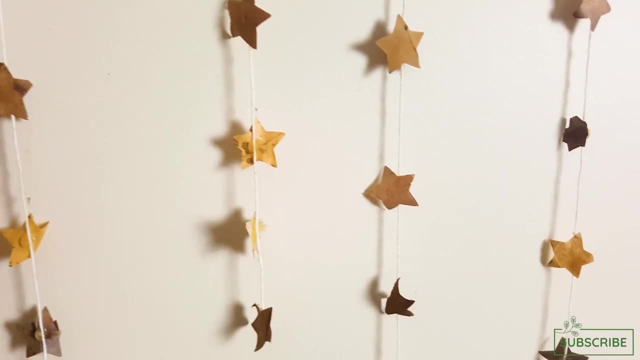 Let's start with materials. Some leaf crafts, stick crafts and rock crafts can last a really super long time. I made this nature star garland, Kidding you. over three years ago I used a star hole punch to cut out the leaves and stuck them on. 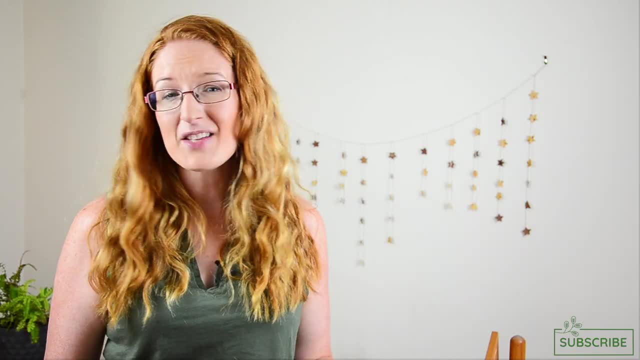 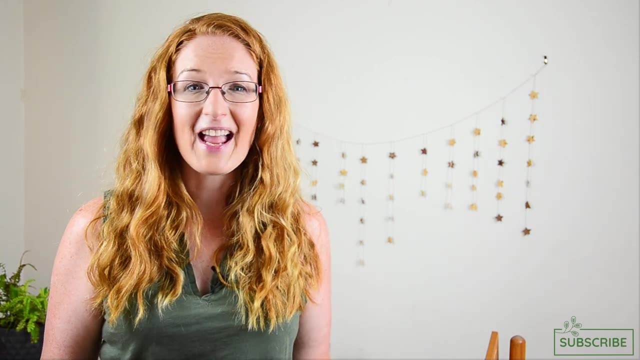 with glue and string and it's lived at my house for about two years and then I took it to my workplace to just jazz up that space where I work, and then I brought it back home. but I didn't use anything on this craft either. They're simply leaves, string and glue. These leaves zombies and 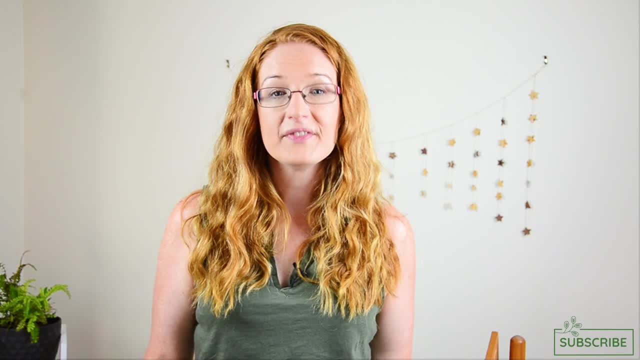 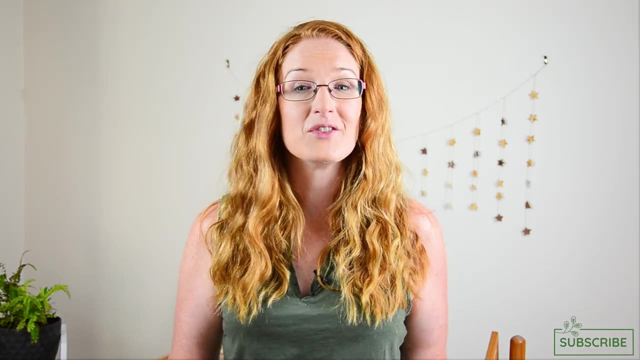 ghosts lasted a couple of years too. Of course, flowers, grass and soft green leaves don't tend to last very long. If they're not pressed and dried up, they're not going to last very long. So picking your natural materials is really important. The glue that you use can impact the 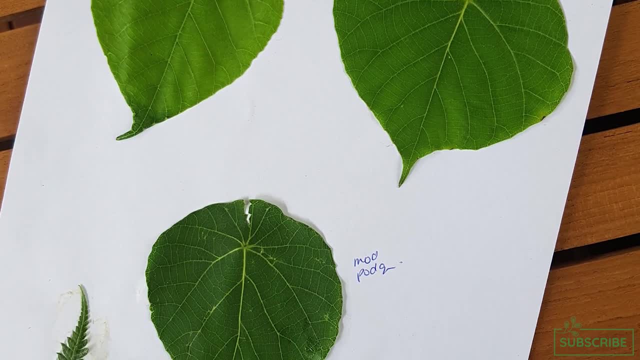 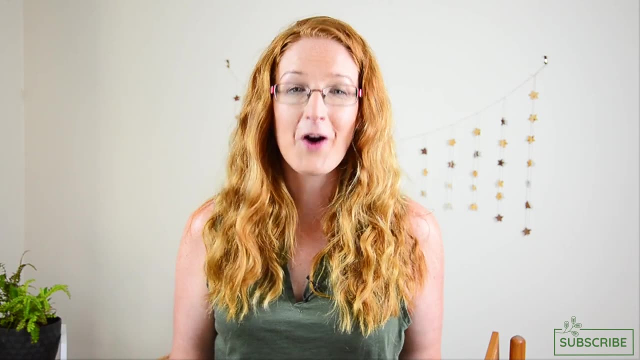 life of your nature crafts. If you're interested in what glue is best for nature crafts, my girls and I did an experiment here, So watch this video and I'd encourage you to do a test with your own children. The environment: As mentioned before, the environment can make a difference to the 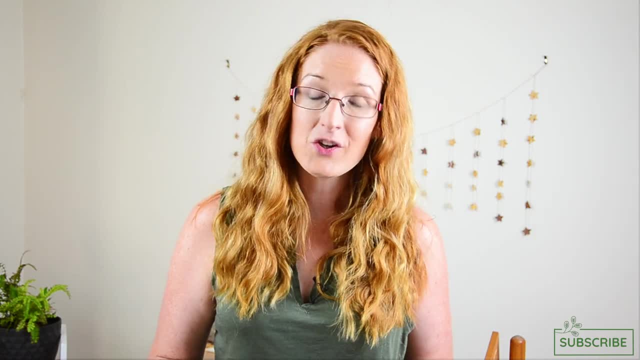 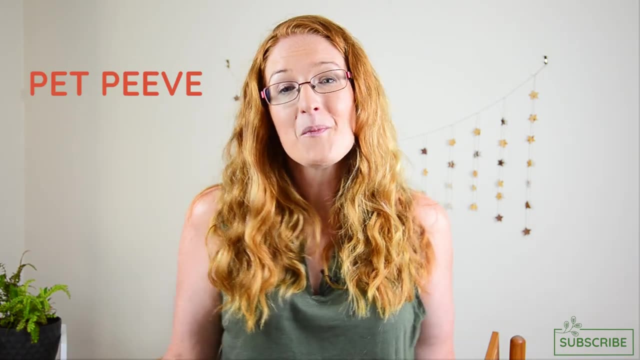 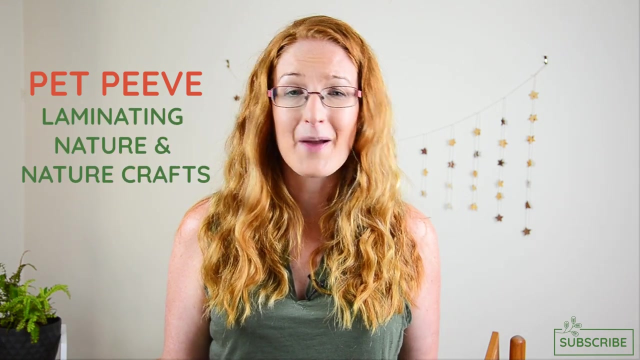 longevity of your nature crafts. They last longer in cooler weather. In summer, our leaves can start curling within 24 hours. Now on to my pet peeve. Now, some of you might already know this, but my pet peeve is laminating nature. Now, don't feel guilty if you've done that before. 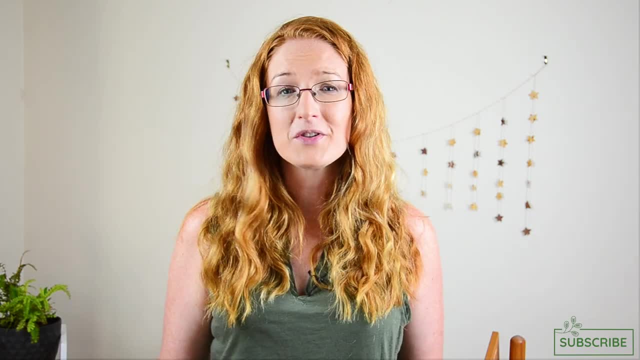 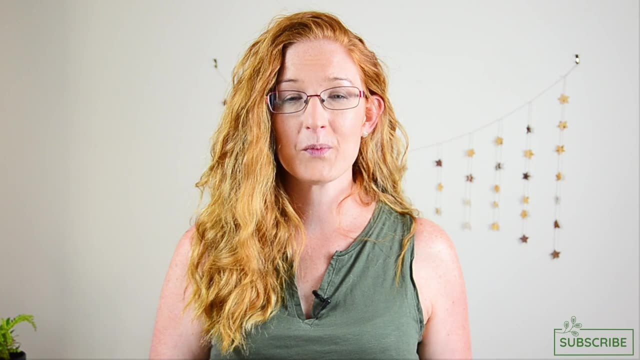 I am not perfect and I'm not 100% sustainable. We're all just trying to get a little better each day, but in my opinion, you do not need to laminate nature, and you shouldn't. Why don't I like it? Well, it turns something biodegradable into something that's not going to biodegrade. 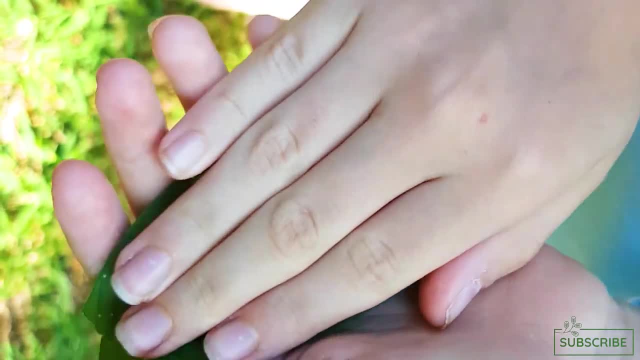 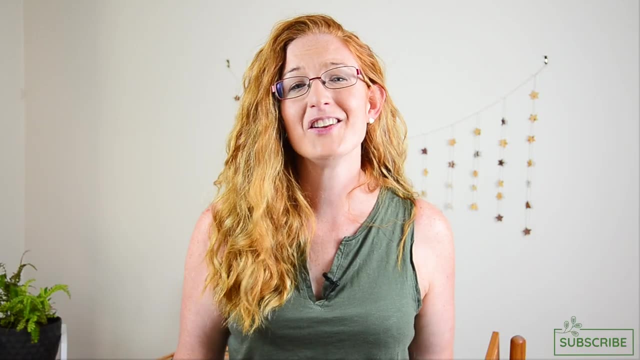 for hundreds of years. Also, another big problem is that it takes the sensory delight out of playing with nature. Now you're just playing with something in case it's not going to biodegrade. You can't just throw it away in the landfill and it's going to be used in plastic, And how long. 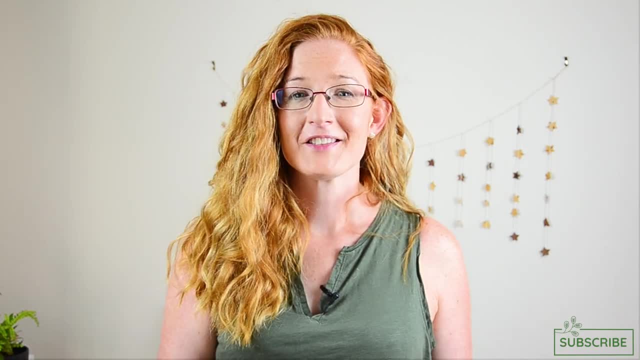 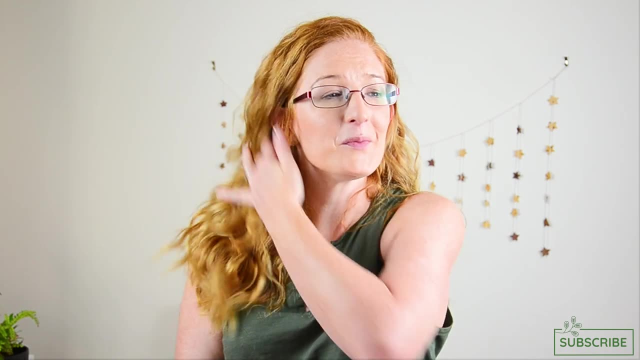 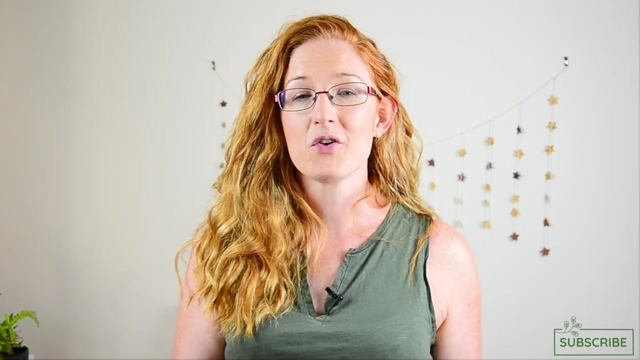 does it take before it's thrown away into landfill anyway? There are other eco-friendly ways to preserve nature. So some of these is using nothing at all. So in my nature crafts I really don't use anything. I don't cover it with plastic, I don't cover it with glue, I don't cover it with beeswax.